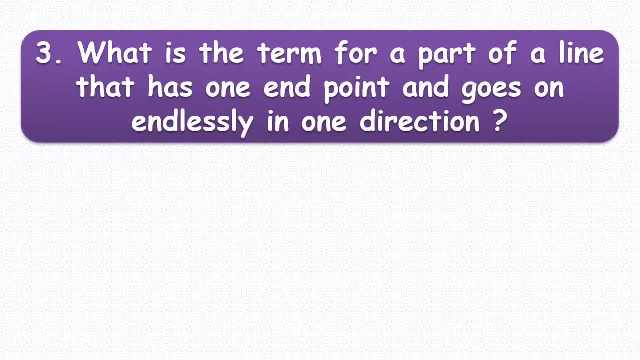 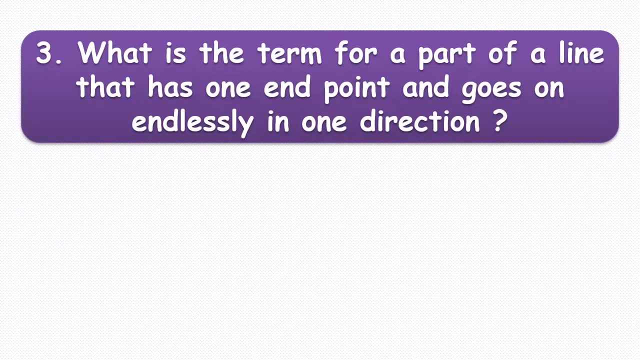 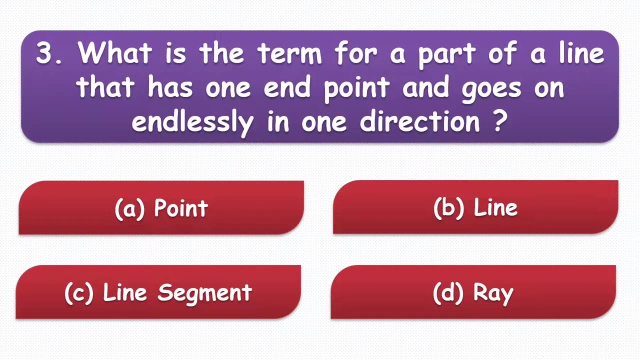 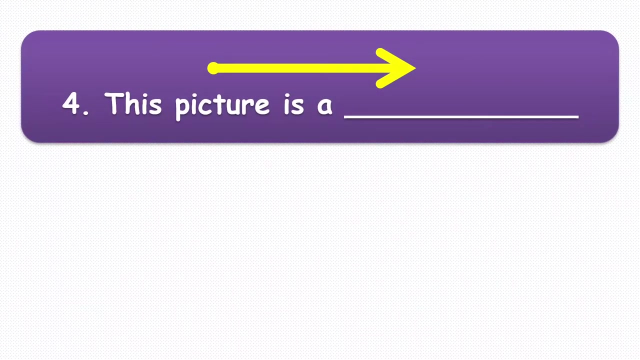 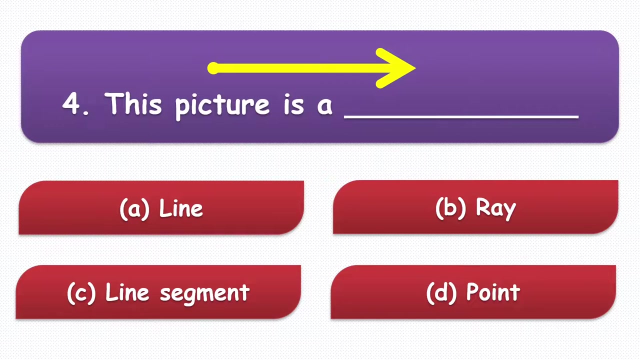 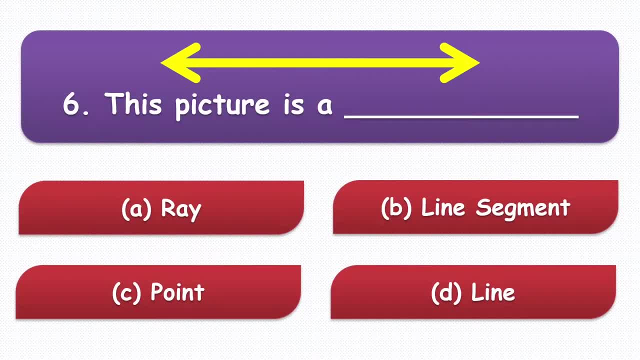 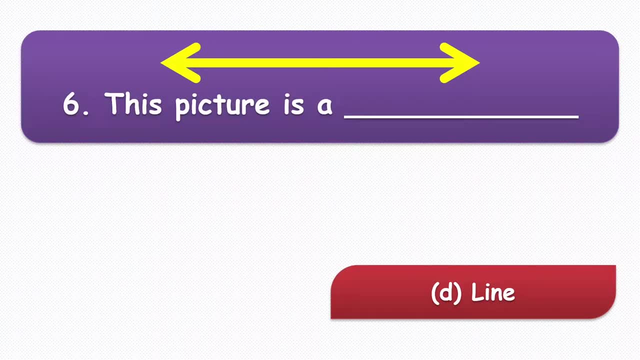 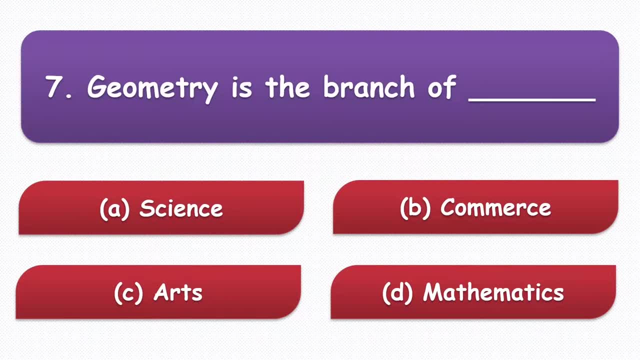 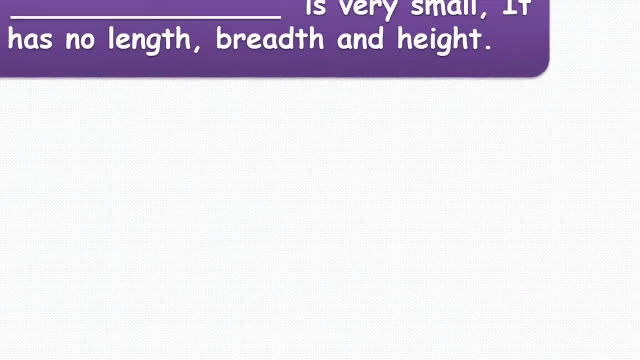 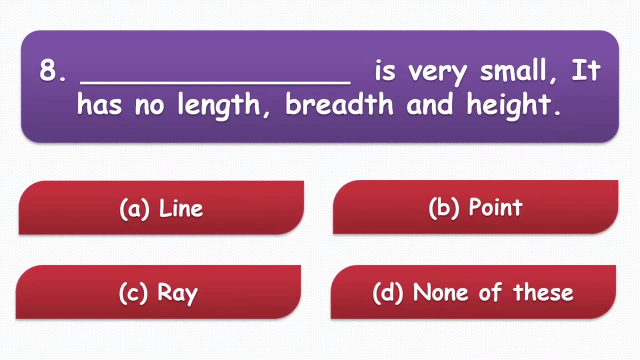 So the options are issue are science, commerce, arts and mathematics. So the correct answer is mathematics. So the correct answer is mathematics. Next question is: Das is very small. It has no length, breadth and height. So the option for this question is line, point ray and none of this. 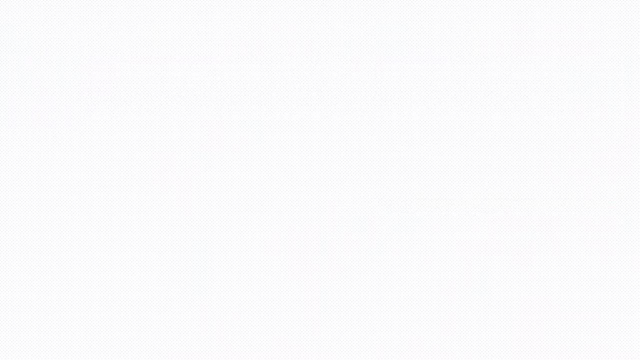 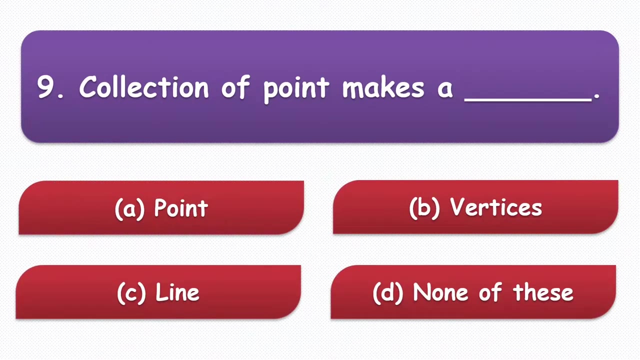 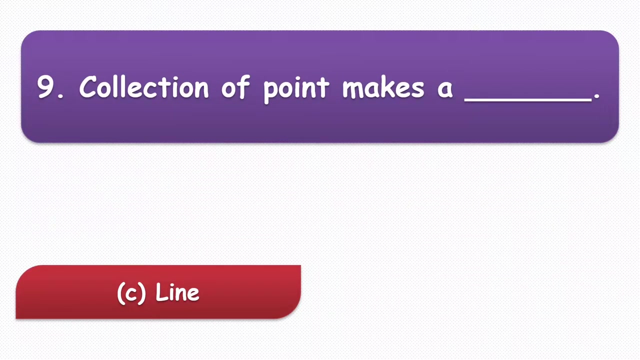 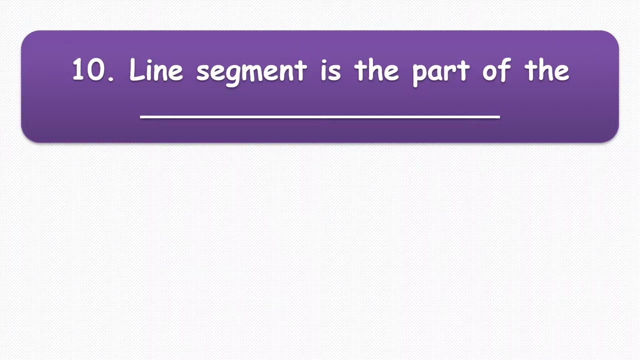 So the answer is point. Next question is: Collection of point makes a das dash. so the options are: point, vertices, line or none of this. so the correct answer for this question is line. next question is: line segment is the part of the dash. so the option for this question is: 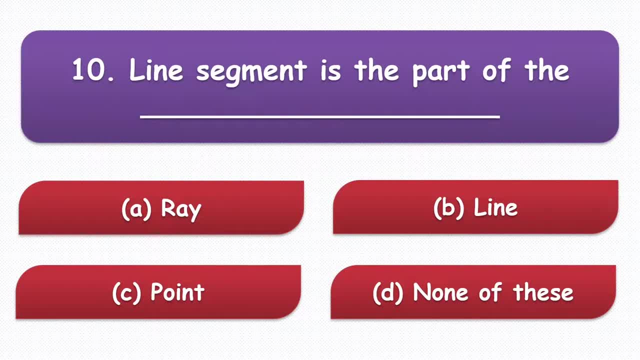 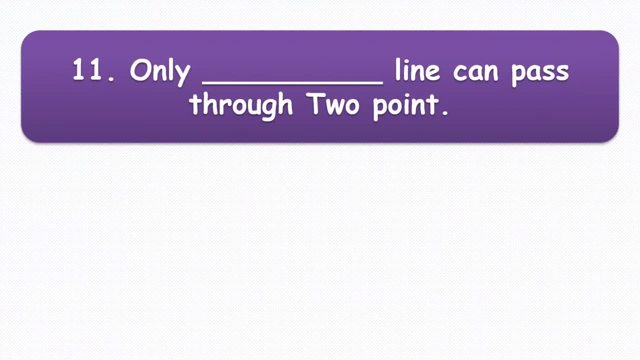 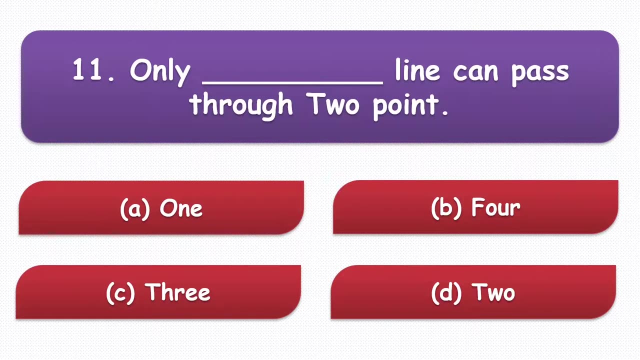 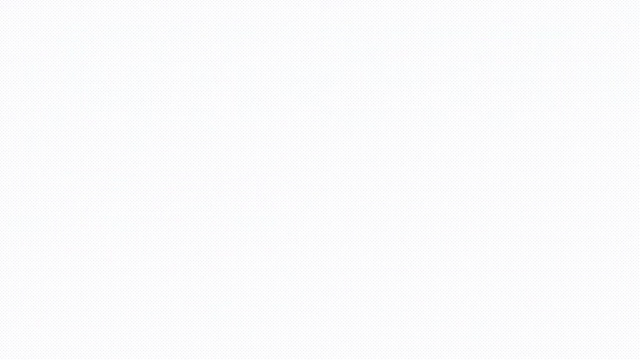 ray line point and none of this. so the answer is line. next question is: only dash line can pass through two point. so the option for this question is one, four, three, two. so the option is: so the answer is one. next question is if two lines meet at 90 degree. 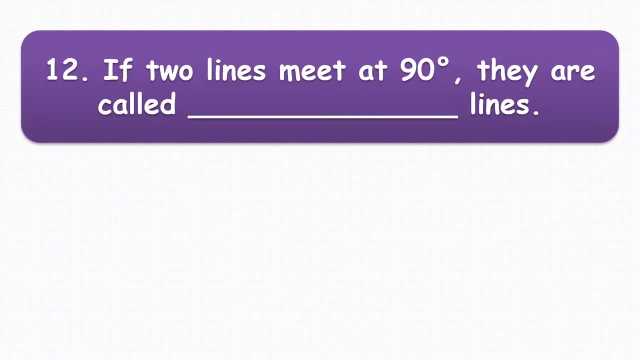 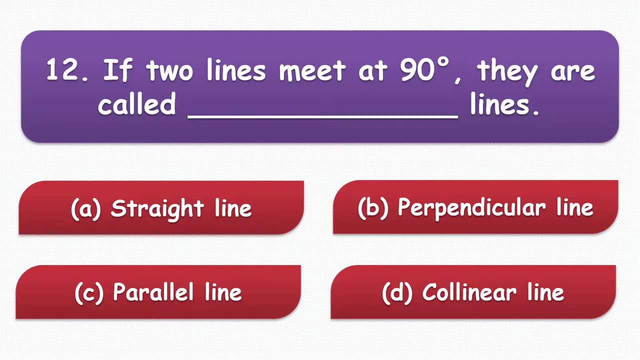 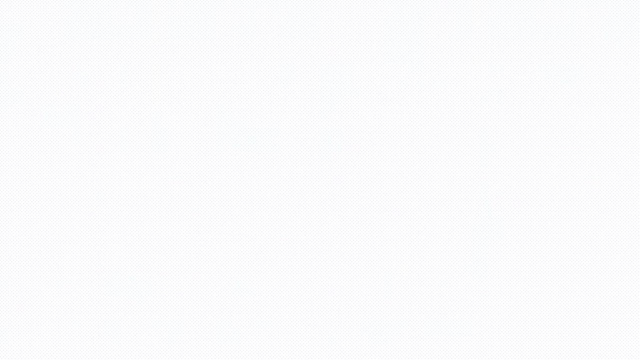 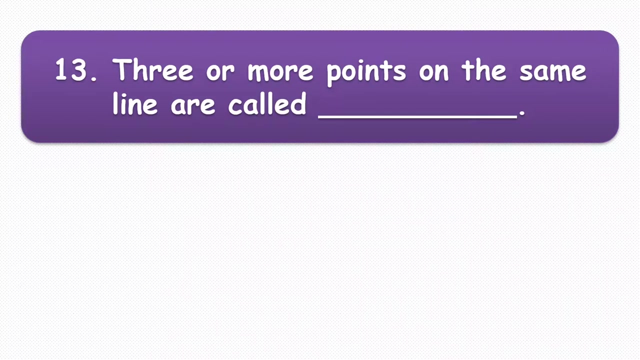 they are called dash lines. so the option for this question is straight line, perpendicular line, parallel line and diagonal line or colinear lines. so the correct answer for this question is perpendicular line. next question is: three or more points on the same line are called dash, so the options are: 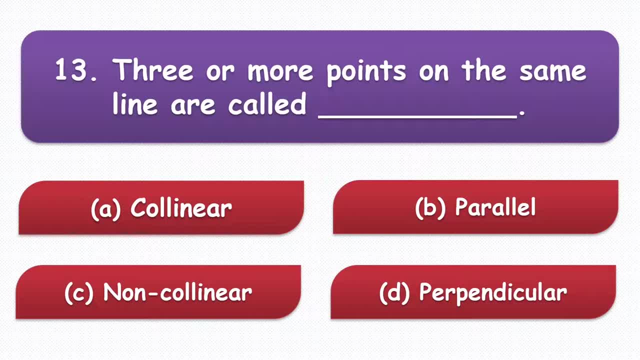 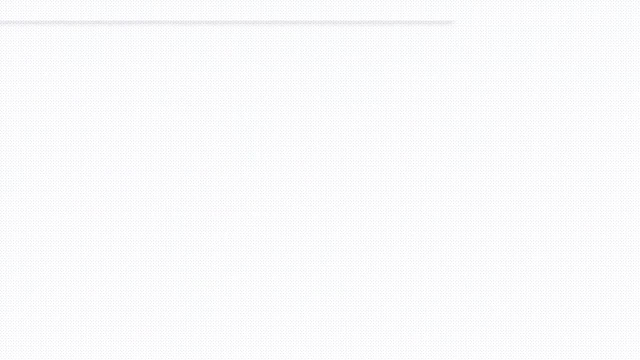 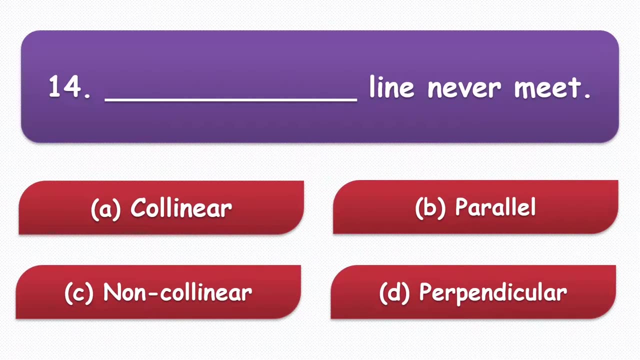 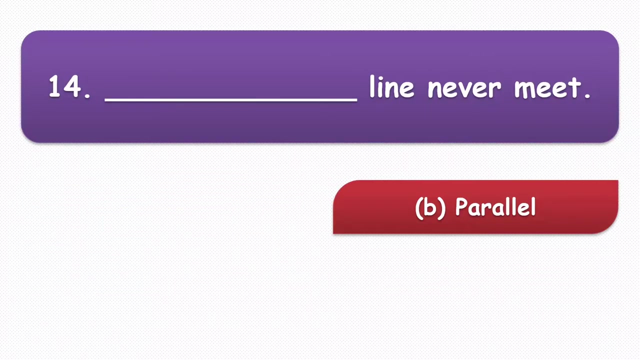 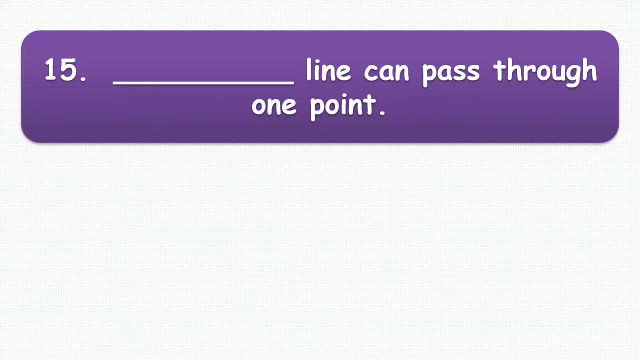 collinear, parallel, non-collinear or perpendicular. so the answer is collinear. next question is: dash line never meet. so the option is: options are collinear, parallel, non-collinear or perpendicular. So the answer is parallel. The last question is: thus: line can pass through one point. So the option of this question. 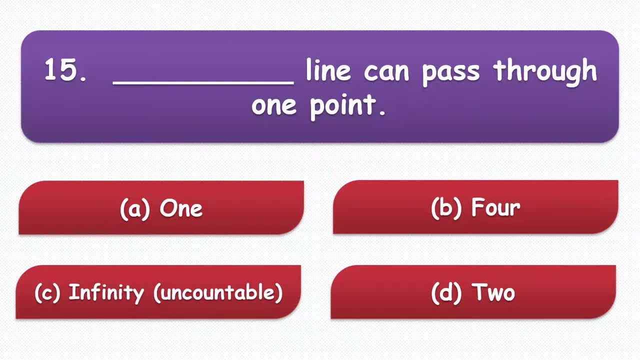 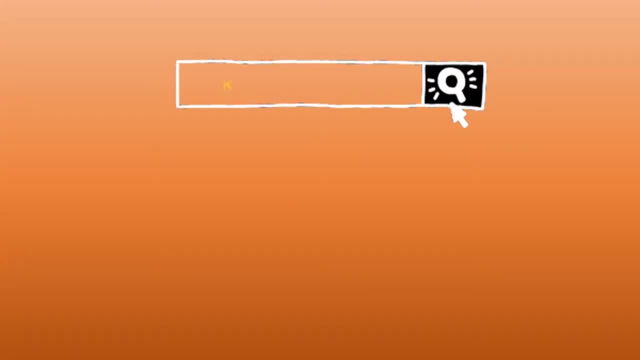 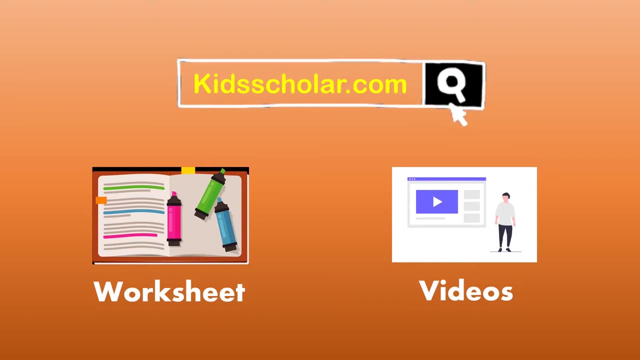 is 1,, 4,, infinity or 2.. Correct answer for this question is infinity, or you can say uncountable. Thank you, 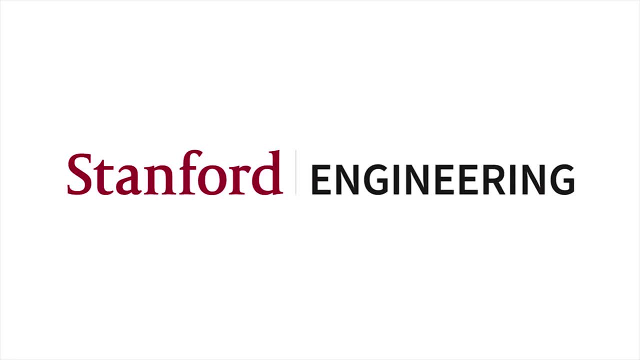 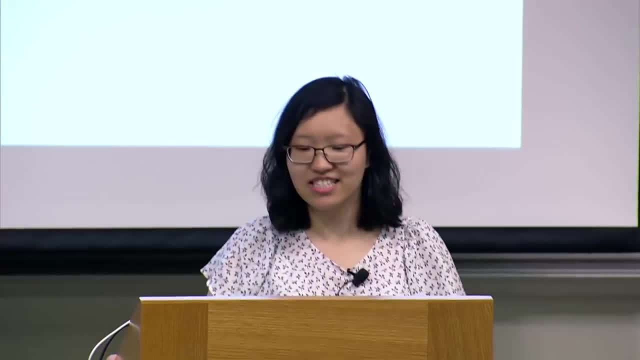 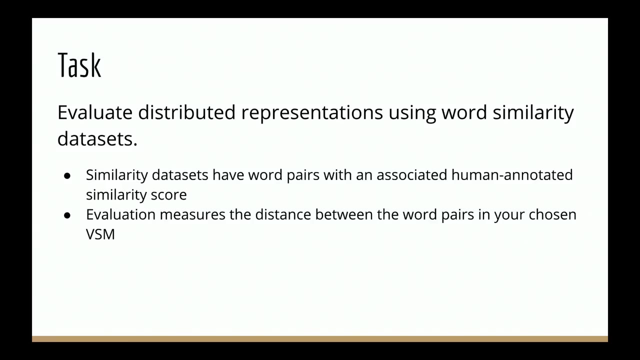 Hi everyone, Hope you had a good weekend. We're going to start off today's class talking about the bake-off that happened last week. So, if you don't remember what you did, you evaluated distributed representations using word similarity datasets, And so all the similarity datasets had these word pairs with associated human annotated similarity scores. 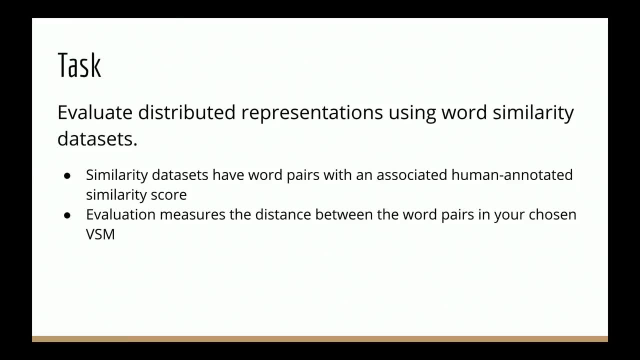 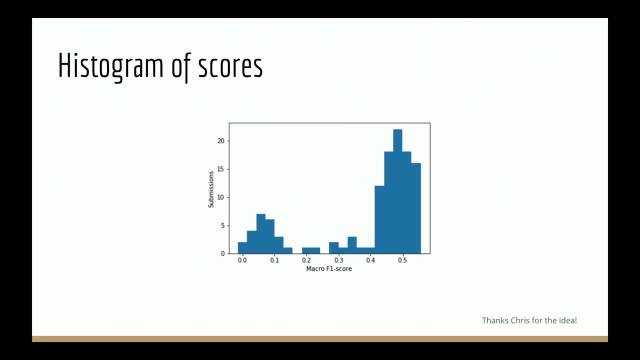 And your evaluation measured the distance between the word pairs in your chosen VSM. So here's a histogram of the scores. As you can see, there's like kind of two bumps: One on the lower end, one on the higher end. Most people were on the higher end. 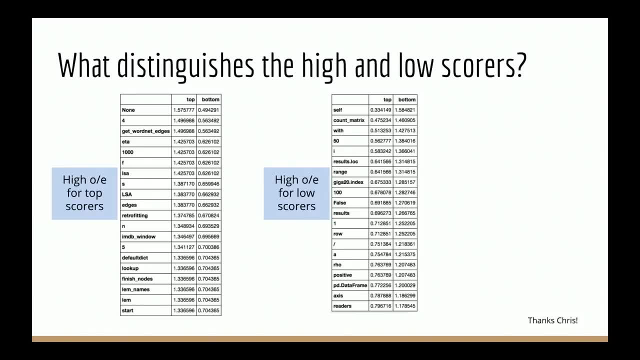 So what Chris did was calculate the observed over expected scores after separating all the bake-off entries into the top scoring teams and to the bottom scoring teams. So on the left here we have the- the words that are like more likely to appear for top scoring teams. 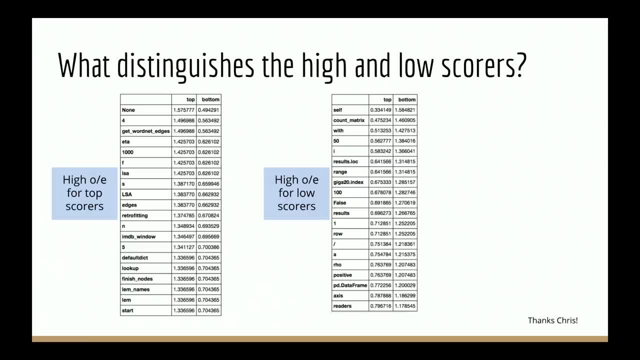 And then over here we have the ones that are more likely to appear for the ones in bottom scoring teams. So that helps you get an idea of like what distinguishes the really good models from the models. So so it seems like retrofitting on WordNet and using LSA are common ways to build better models from this rough analysis. 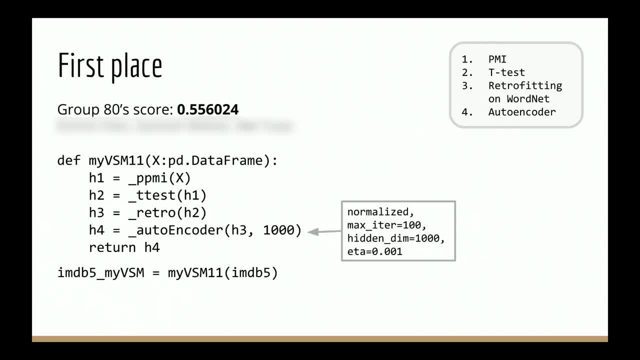 Okay, So our first place team is group 80.. Is group 80 here? No, Okay, But yeah, group 80, basically stacked PP-, PP-, PPMI t-test, retrofitting on WordNet and an autoencoder.